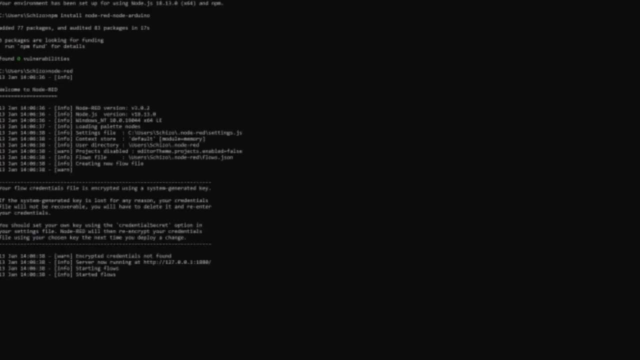 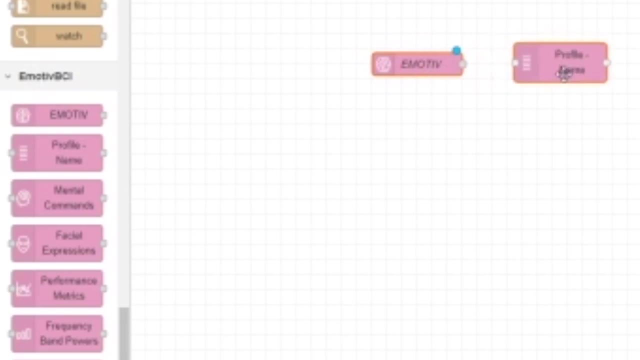 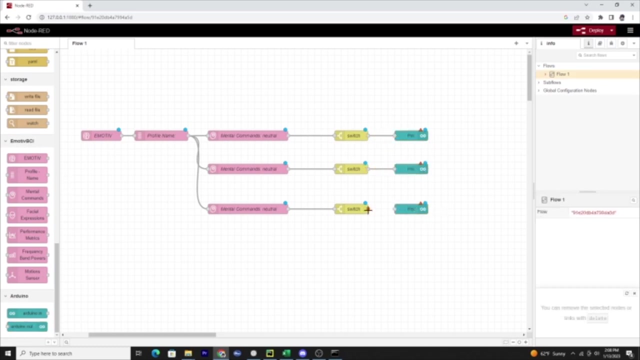 a more physical effect, as you can program computer-controlled electronic devices. To demonstrate, I made this basic block code on Node-RED which takes training profiles from my Emotive app and applies the commands from that profile to activate different colored LEDs. The more commands you add, the less efficient this becomes, but it's nonetheless. 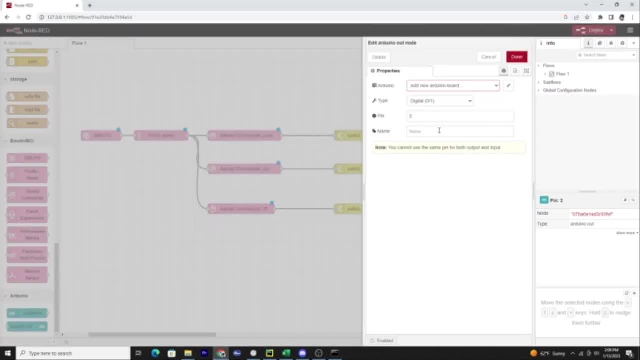 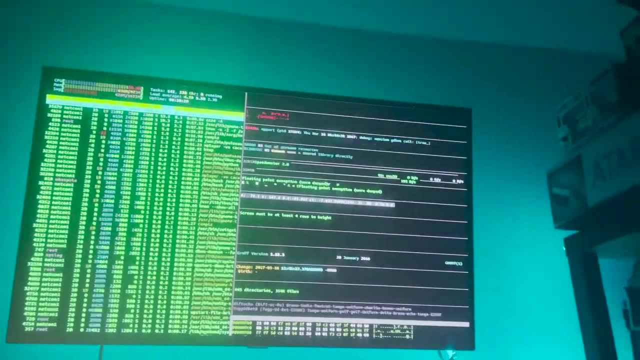 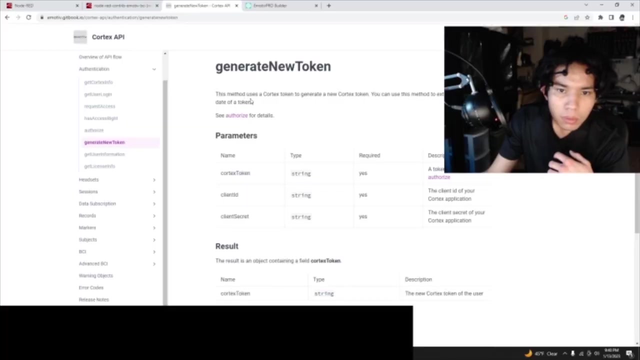 a cool technology that you can use to control anything from computer commands to servo motors, And, as much as we all want coding a brain-computer interface to look something like this: Here's a condensed version of the nightmare that actually occurred, as I low-key sometimes. 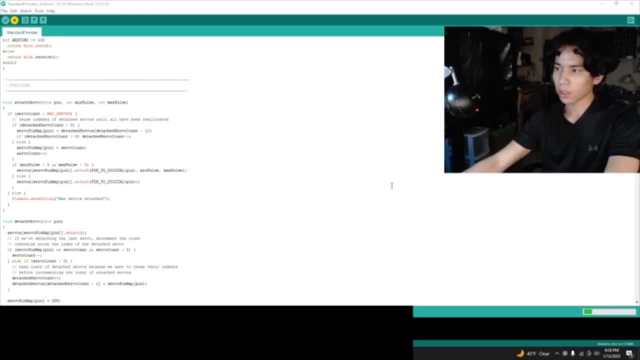 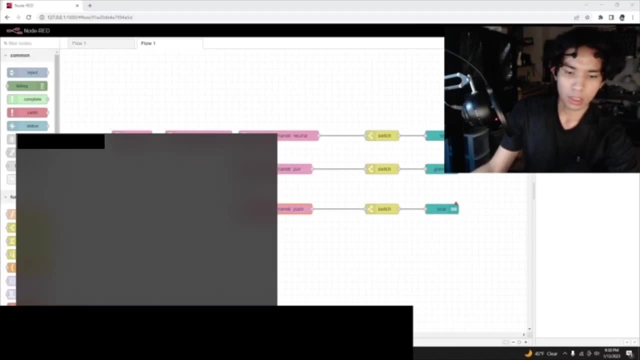 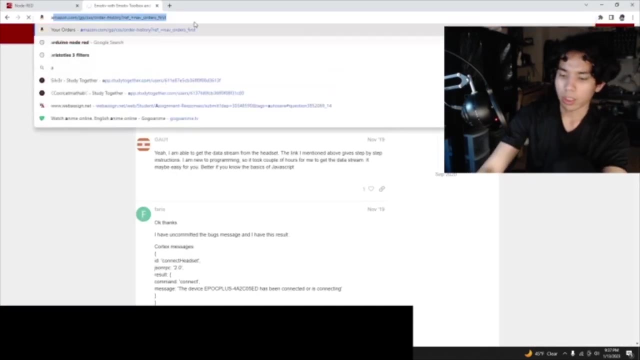 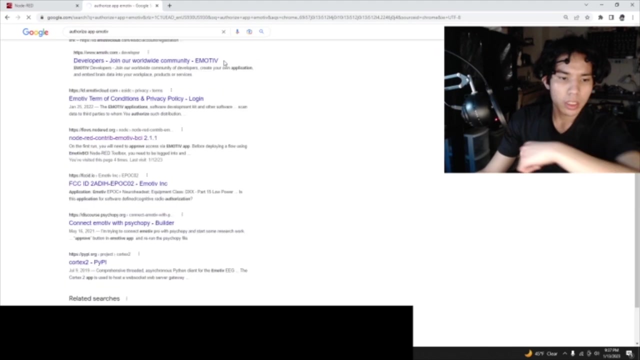 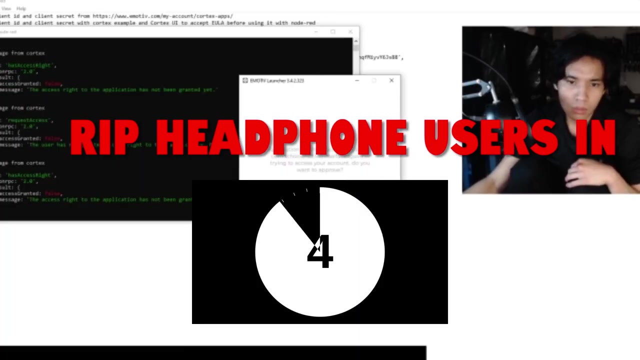 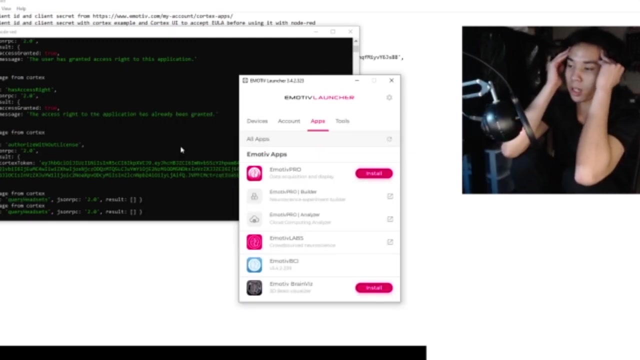 can't program for shit. Okay, right now I'm uploading the communications protocol to the Arduino. Oh, my headset Duh Forgot. I have to authorize the app. Right, there's an authorization process Many hours later, God, finally. Thank you, Jesus Christ. That took way too long. 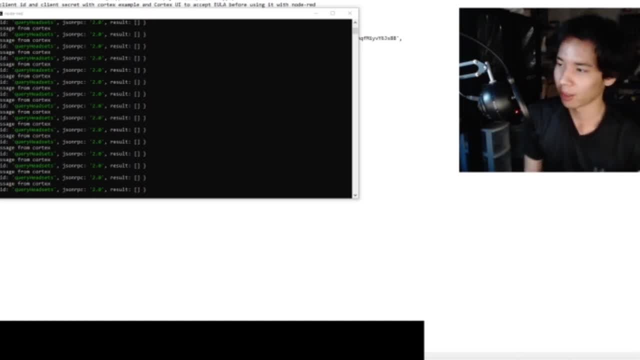 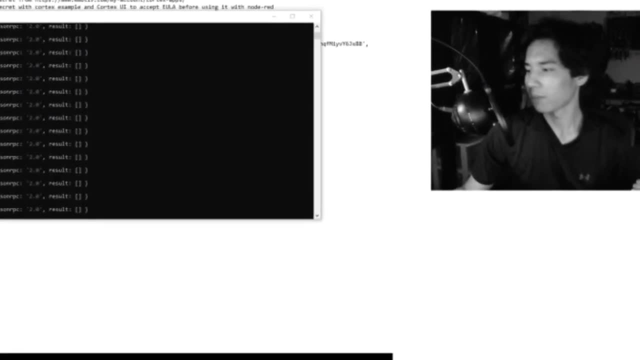 Well, it's not over yet, because now I have to wait for my headset to finish charging. It practically died while I was doing that. Me from 16 hours ago has no idea how correct he actually is. It was indeed not over, and he would spend the next several hours trying to figure out. 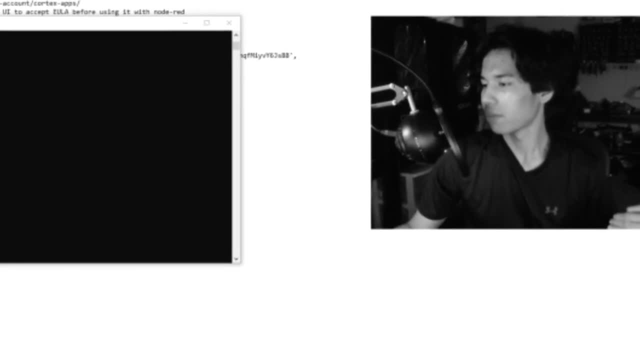 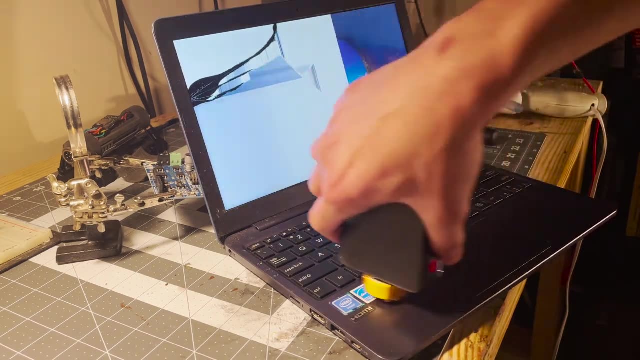 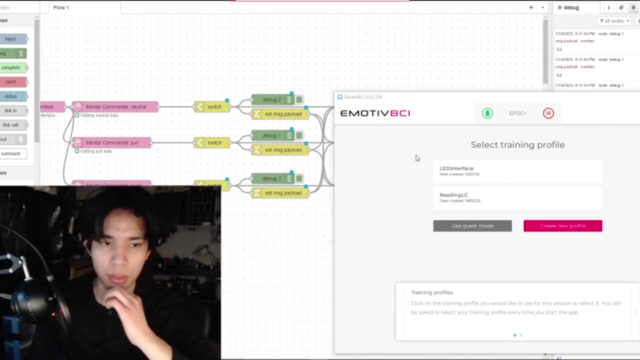 how he activated the microcontroller pins. three years ago I used to have a laptop with the original nodes, but Now I don't The next day. Alright, the way I have things set up right now, The red LED is linked to the neutral command. 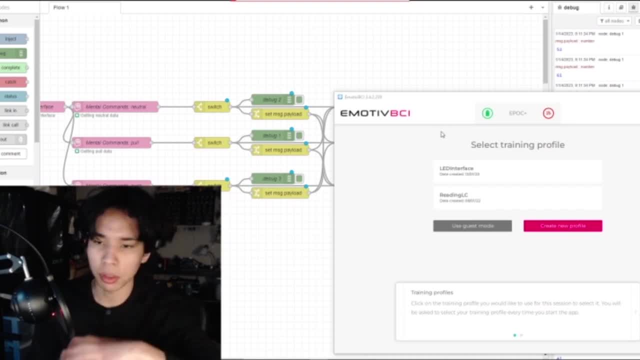 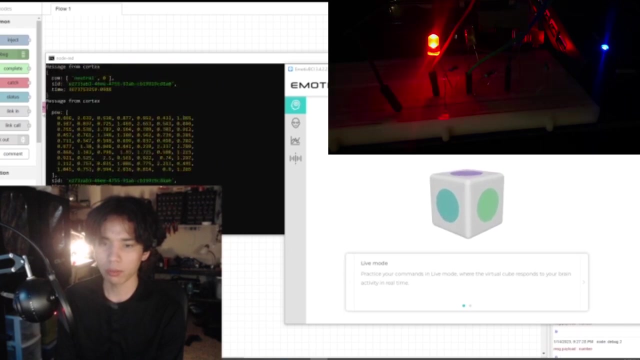 The green LED is linked to the pull command And the blue LED is linked to the push command, So hopefully all goes well. Start the LED camera: Red, Green, Blue. As you can see, there is some inefficiency with interpreting the EEG commands.